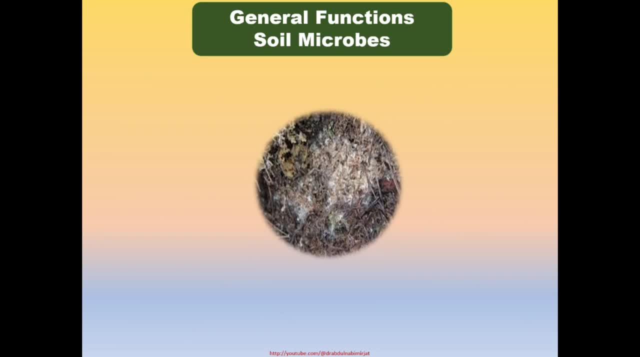 General functions of soil microorganisms. Soil microbes play an important role in soil, Such as decomposition, nitrification, nitrogen fixation and denitrification and even many more other functions. Mainly the decomposition of various kinds of organic matter and plant and animal material is one of the major role played by soil microorganisms. 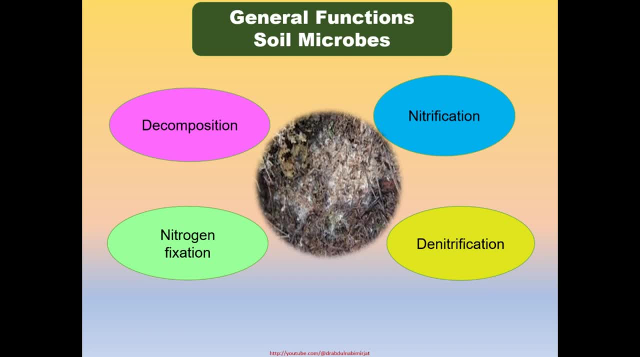 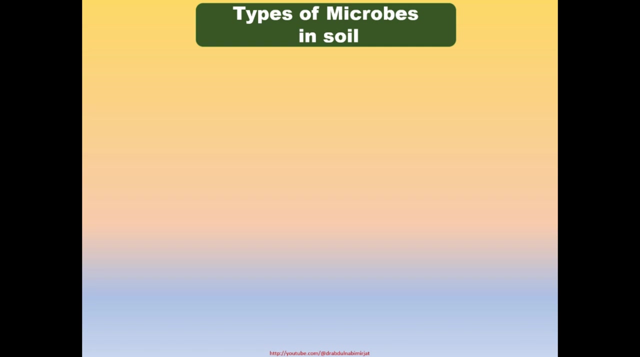 For the transmission of chemical substances that can be utilized by soil microorganisms. Soil microorganisms serve as the biochemical agents for the conversion of complex organic compounds into simple inorganic compounds. Types of microbes in soil. Several types of living organisms are found in soil. 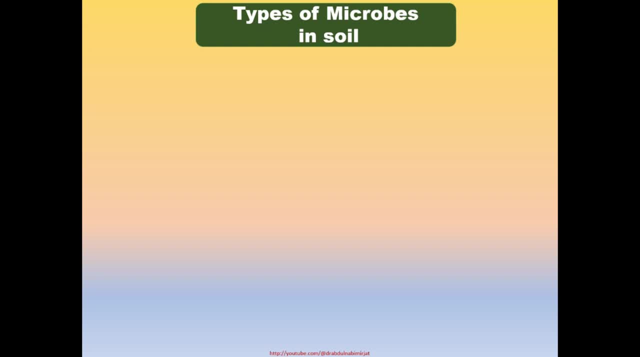 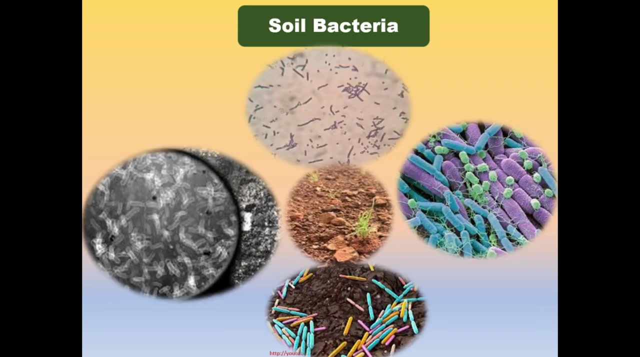 However, there are five major groups of microbes found commonly in soil, Such as bacteria, actinomycete, fungi, algae and protozoa. Soil bacteria. Bacteria are the smallest and free living population in soil. Bacteria are considered as the most important soil microorganisms due to their size and simple morphology. 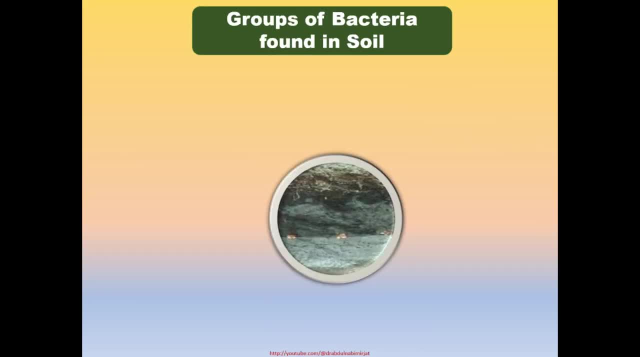 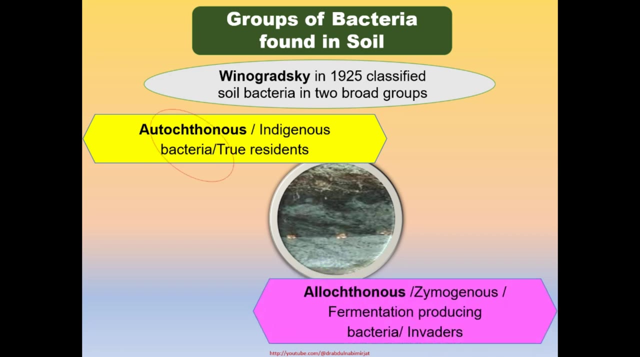 Groups of bacteria found in soil. Vinogrovsky in 1925 classified soil bacteria into two broad groups, Such as autochthonous and allochthonous. Autochthonous soil bacteria are known as the true residents in soil. These are long survival and help in biological functions. 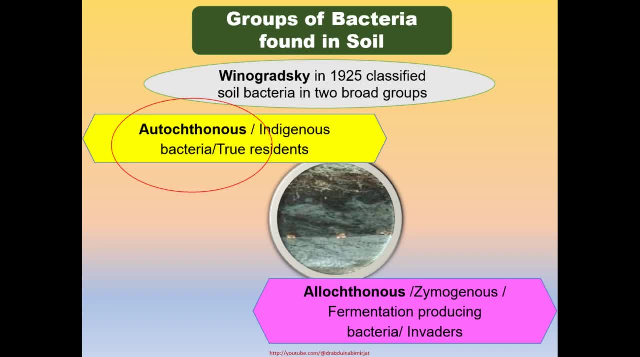 These types of bacteria derive their nutrients from organic fraction of the soil, but no any external source of energy, Whereas allochthonous bacteria they are called as zymogenous or fermentation producing bacteria. Even they are also called as invaders. They are less in quantity as compared to allochthonous. 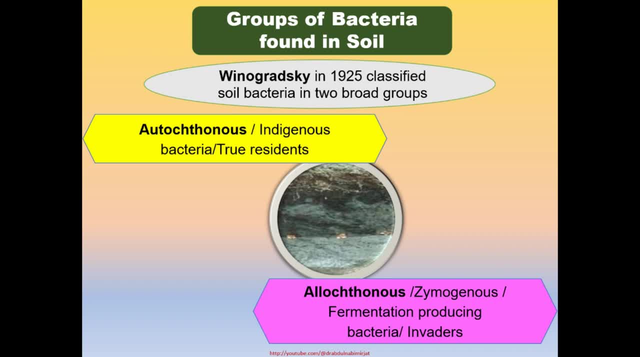 They are less in quantity as compared to allochthonous Substrate is needed to perform chemical transformation. They require external source of nutrients for energy. The population or growth increased after addition of organic material in soil And with exhaustion of organic nutrients their growth decreased rapidly. 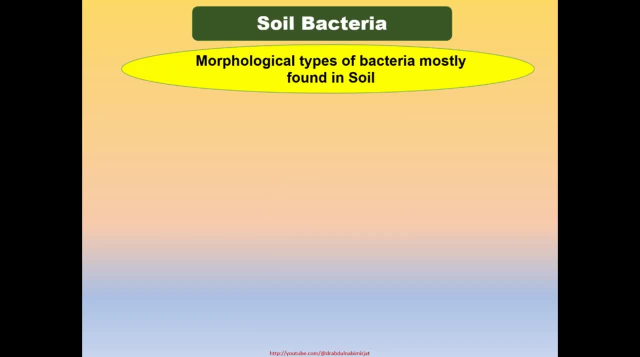 Morphological types of bacteria Mostly found in soil, Such as coxae, bacilli and spirula. The bacteria with coxae morphology are not in common in soil, Whereas the bacilli are found as most numerous due to endosperm formation. 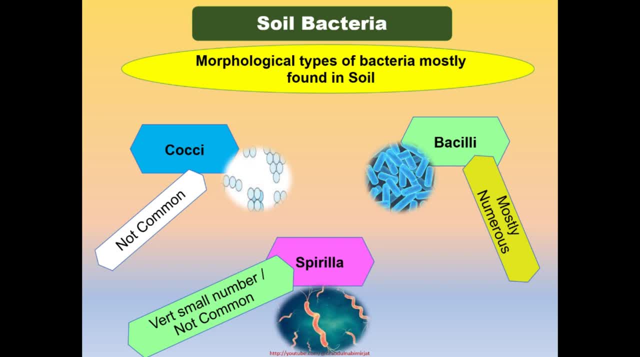 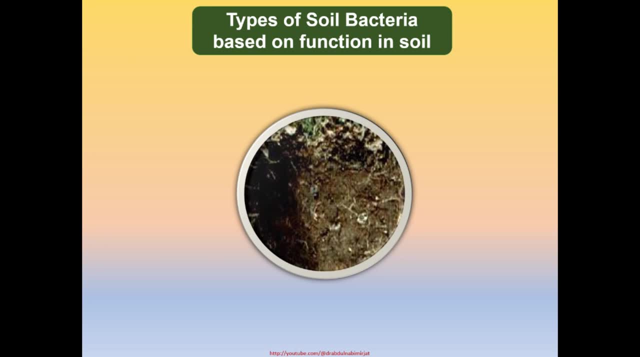 While spirula are found in various forms, Spirula are found in very small number in soil. Types of soil bacteria Based on functions in soil. Soil bacteria play an important role in soil. These bacteria produce different types of the extracellular enzymes. 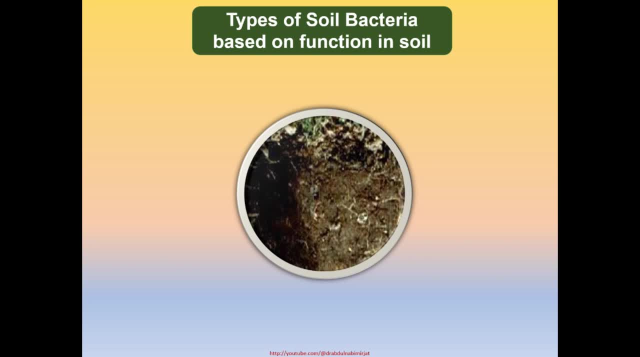 Such as amylase, protease, lipase, phosphatase And even many more other extracellular enzymes. Also, soil bacteria produce antimicrobial substances. So, based on different functions, These type of the bacteria are classified into several groups, Such as decomposers. 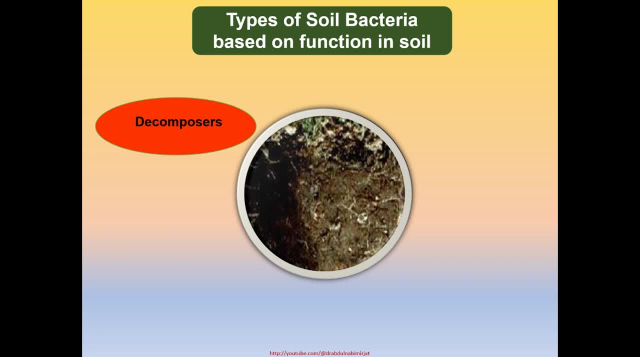 Which play an important role in decomposition of organic matter. Nitrogen fixers: These bacteria extract nitrogen gas from air And convert it into different forms used by plants. Among the nitrogen fixers, The nitrobacter species are known as the nitrogen fixers. 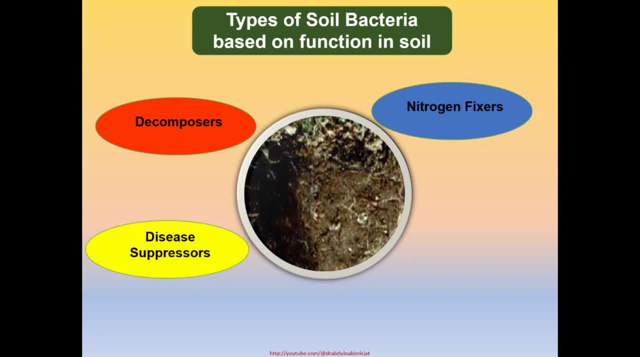 Another group called as disease suppressors. These type of the soil bacteria release antibiotic substances To suppress the growth of other bacteria or particular competitors. Actinobacter. Actinobacter. slowly break down humic acids in soil. These type of the bacteria prefer non-acid soils with more than 5 pH.